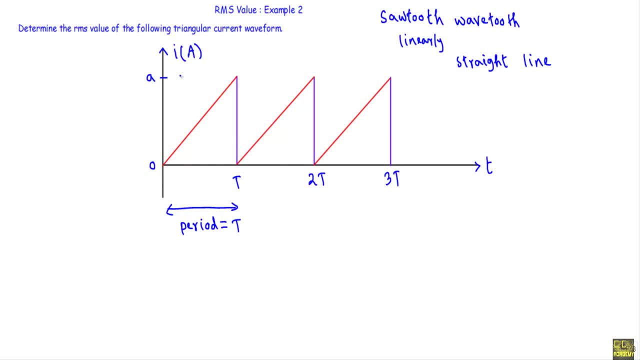 That means we can express the change from 0 to t interval of the current using the standard straight line equation: y equal to mx plus c. Here the current is going through the origin. As a result, the y-intersect will be equal to 0.. 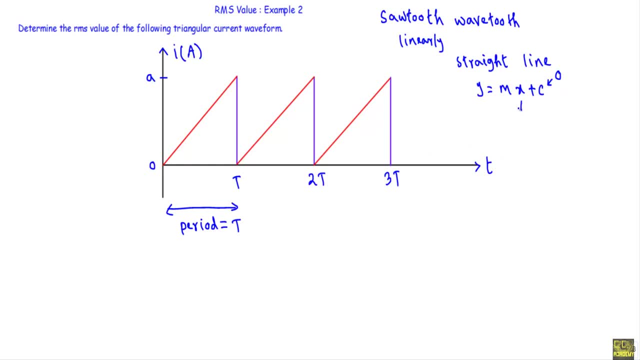 Now see: in the x-axis we are taking time t, so x variable will represent time, and in the y-axis we are taking current i. Now we have to calculate the slope of the equation and the slope will be equal. to see, this is our origin, so it will have coordinate of. 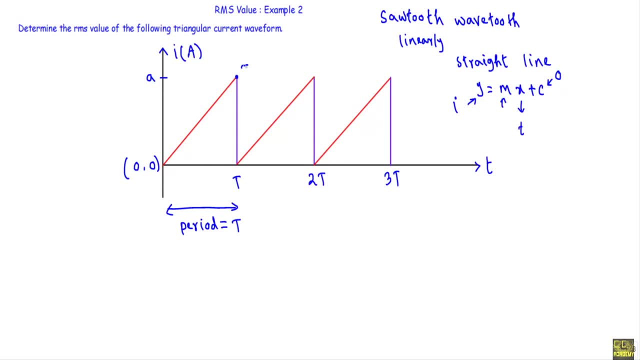 This point has its x coordinate t And y coordinate a, So this point will have a coordinate of. Now how do we calculate the slope of a straight line? Slope is expressed with: m Change in y-axis y2 minus y1 over change in x-axis x2 minus x1, or rise over run. 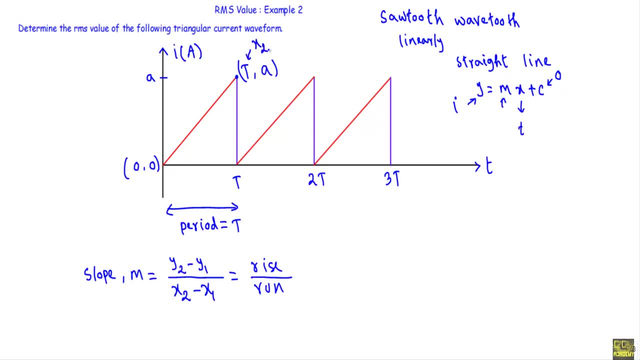 Here this t will express t. Now, if we divide the slope of a straight line by x2, this will be y2.. This will be x1 and this will be y1. So if I use y2 minus y1, divided by x2 minus x1 formula, then I will get busa of a minus. 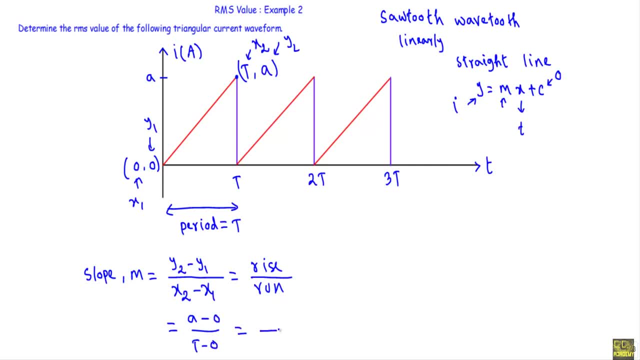 0 over t minus 0, equal to a over t. Therefore, the slope of the straight line m will be equal to a over capital T. Therefore, this slope is equal to m And this is a straight line and if you see, we can write a straight line. 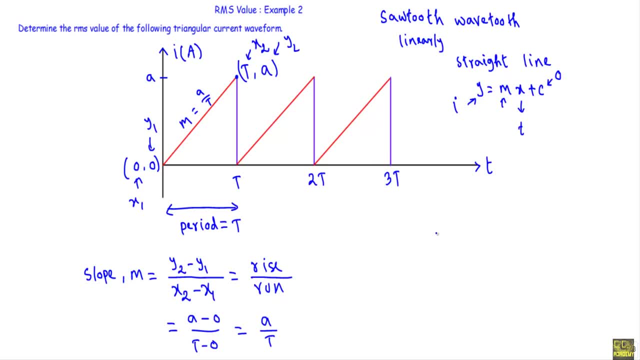 Therefore the slope of this straight line, m is equal to a over capital T. Therefore this is y2 by x2, divided by x2 minus y1.. straight line will have equation of I equal to a over capital T get multiplied with T so we can express this triangular waveform with this time. 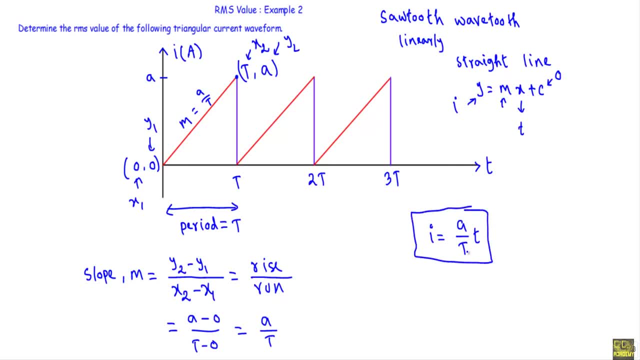 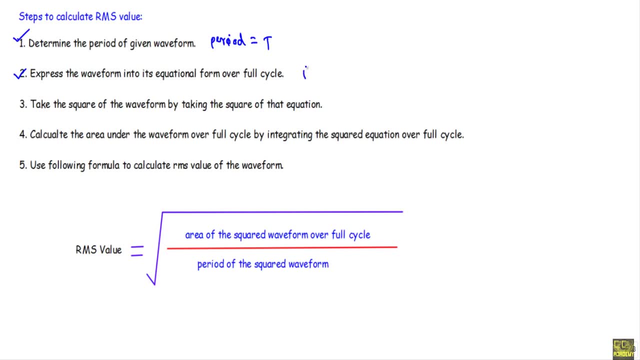 varying equation- I equal to a over capital T into small t. so we get the equation of current I is equal to a over capital T. get them, get multiplied with small t. after that we will take the square of the waveform by taking the square of that equation. see this: I equal to a over capital T into T. 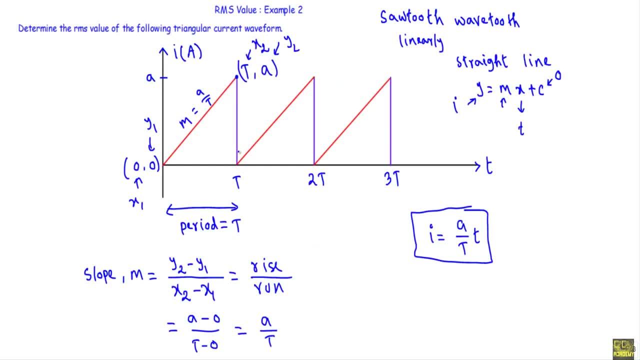 represents this triangular waveform. if I want to take the square of this equation triangular waveform, how do we get that? if I take the square of the alternating quantity, I square, T square, I will get the square of this triangular waveform. therefore, I will get a square over capital, T square, into small t square. so 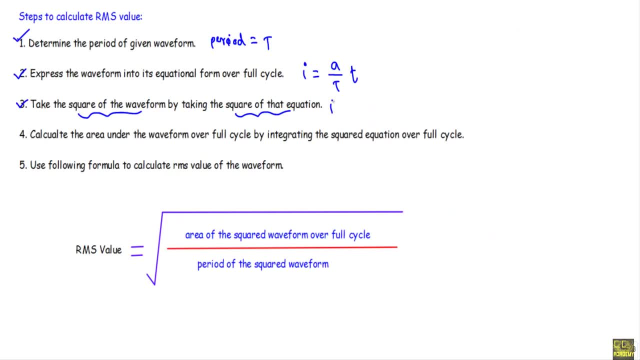 the equation of the squared waveform, of the triangular waveform, will be equal to I square, equal to a square over capital T square into small t square. okay, after that I will calculate the area under the waveform, area under the e squared waveform over full cycle, see RMS value. 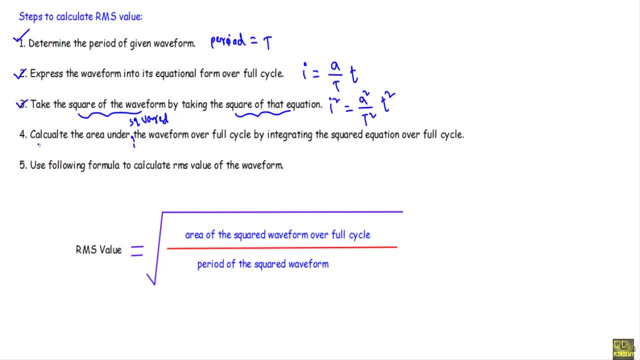 is equal to area of the squared waveform over full cycle. therefore, we will calculate the area under the squared waveform over full cycle by integrating the squared equation over full cycle. see here, our squared equation is I square. if I take the integration of I over a full cycle here, over a full cycle, I will get the interval 0 to T, I will get the area. 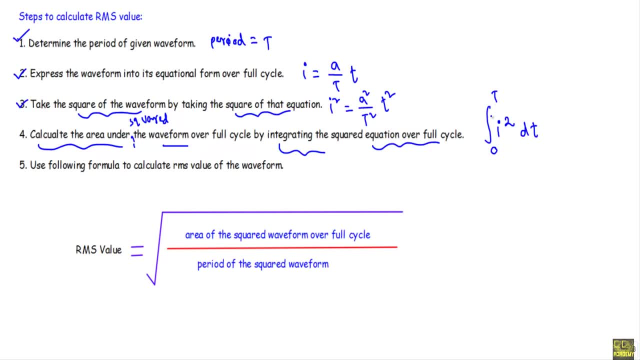 under the squared waveform over full cycle. therefore, this integration of 0 to T I squared DT will indicate the area of the squared waveform or squared current over full cycle. after that we will use this formula: RMS value of current I RMS will be equal to. from the fourth point, we will calculate the area under this: